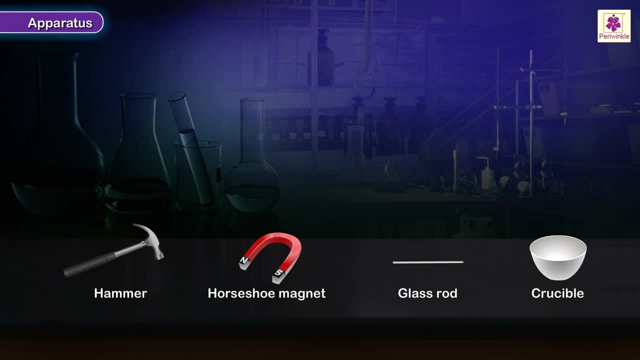 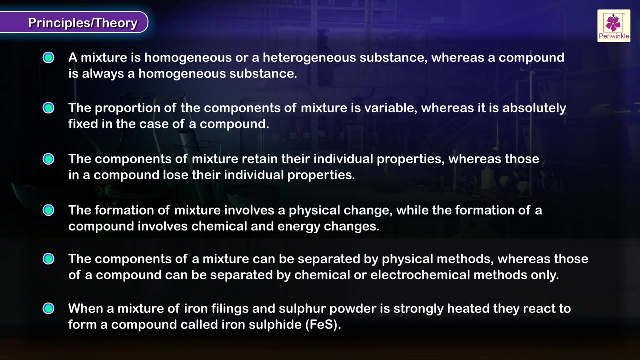 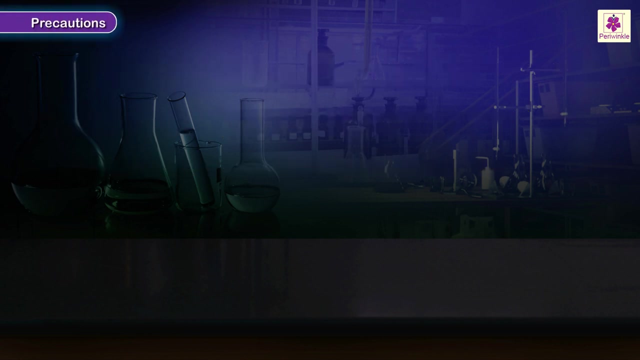 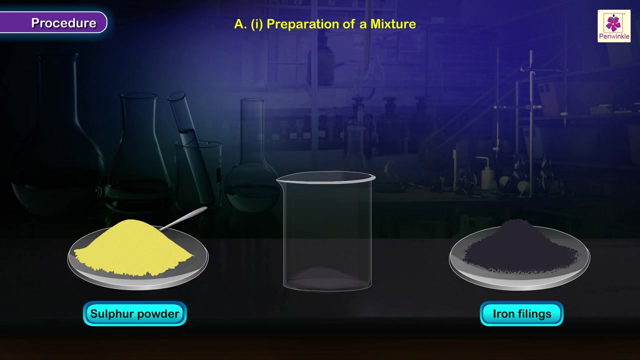 apparatus, chemicals and materials, principles or theory notes, precautions procedure. procedure for the preparation of a mixture of a mixture of a compound procedure. procedure for the preparation of a mixture of a compound. procedure. procedure for the preparation of a mixture of a compound. A woman at two months. she observed a mixture of two particles of a mixture of iron filings and powdered sulphur. 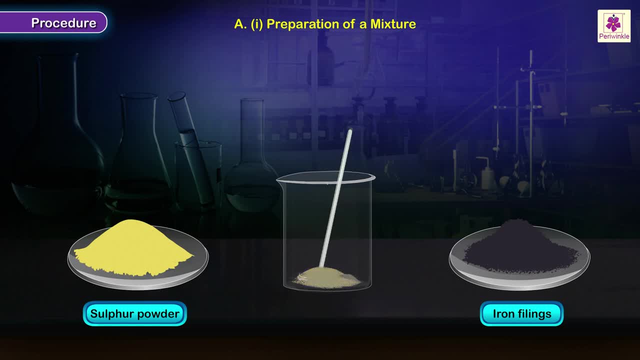 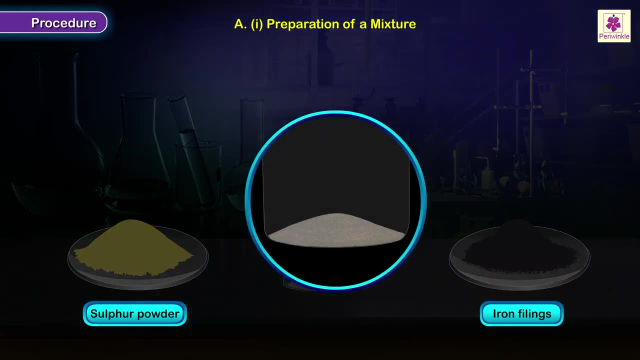 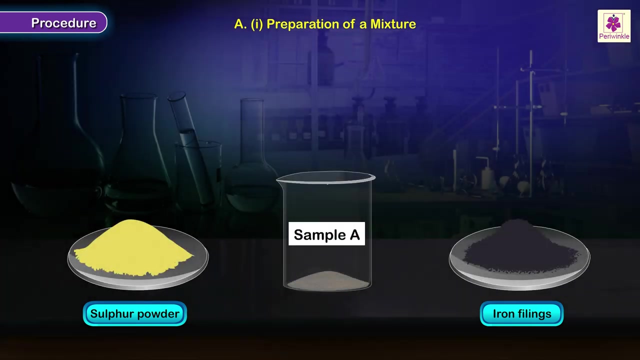 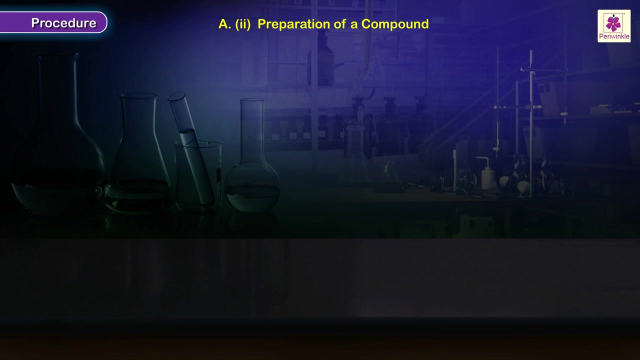 A human being. everyone had in behavior. 속ban проис rutine would be aroundnight relative 수�iscern을 하지만 ready. label this as sample. a procedure for the preparation of a compound of iron and sulfur. take about four to five spoons full of sample a in a clean 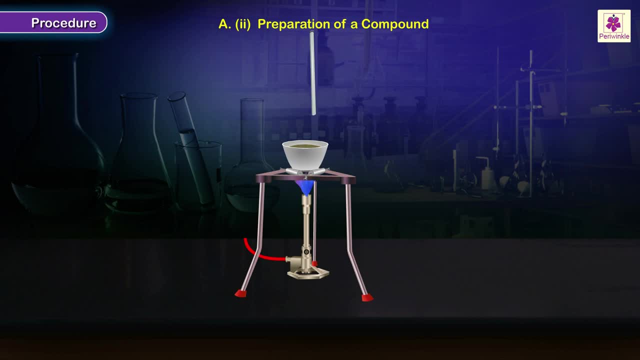 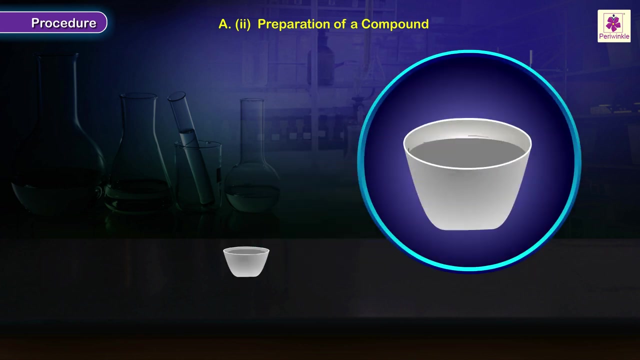 crucible. strongly heat the crucible over a gas burner and simultaneously stir the mixture while heating it. stop heating when the mixture turns into a grayish black mass in the crucible. this mass is a compound called iron sulfide. the reaction can be symbolically represented as iron plus sulfur gives. 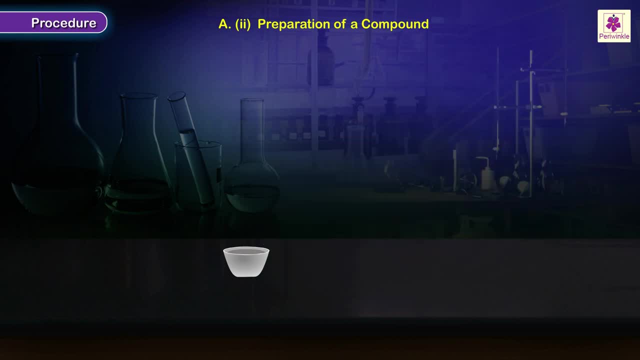 iron sulfide. when the mass cools, remove it from the crucible and place it in a thick cloth bag. found the mass using a hammer to obtain its powder. collect the finely powdered iron sulfide in a clean beaker, labeled sample. be procedure to distinguish between a 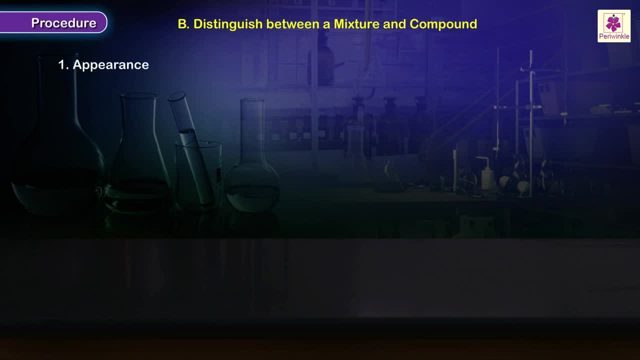 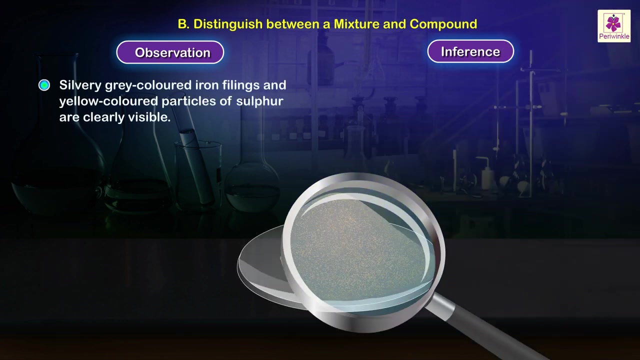 mixture and compound on the basis of their appearance. take a spoonful of sample a on the clean watch glass. observe the mixture with the help of a magnifying glass. observation and inference. silvery gray colored by filings and yellow colored particles of sulfur are clearly visible. the mixture. 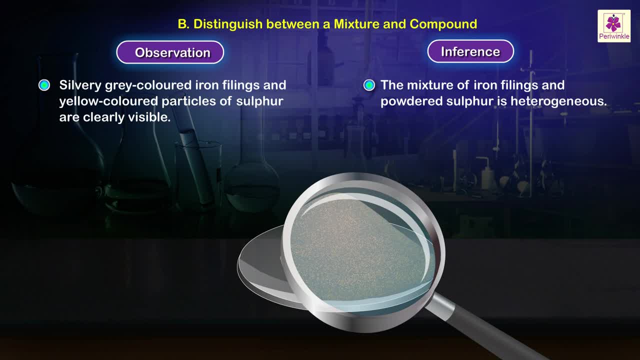 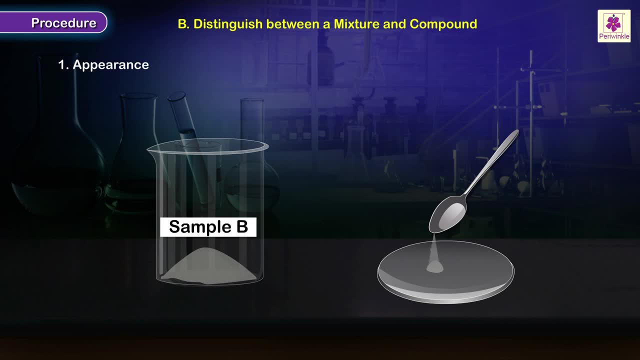 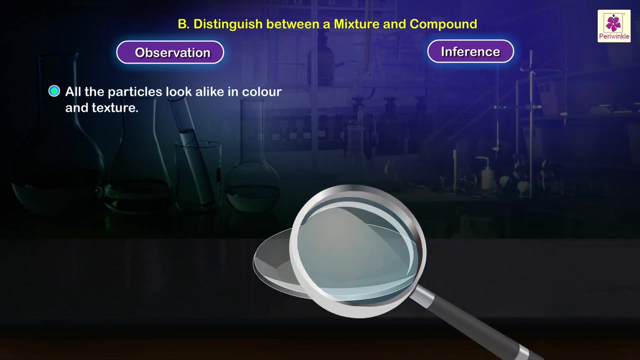 of iron filings and powdered sulfur is heterogeneous. ładae: take a spoonful of sample being on a clean, dry watch glass. observe the particles with the help of a magnifying glass. observations and inference. all the particles look alike in color and texture. iron sulfide is a homogeneous 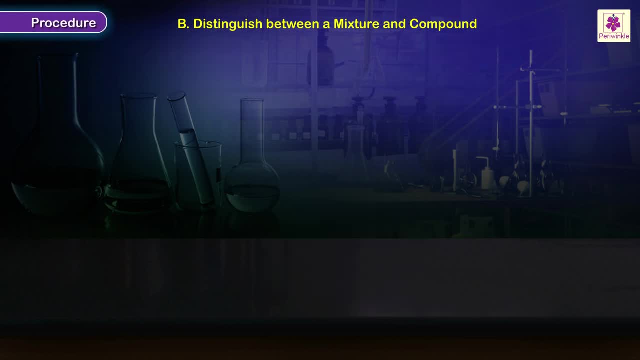 substance. next we will introduce an example of lamaze cellophane. yourselves proced disregardor as the 210 defined one, try to be longing for blood untouched sample whenréal��� to distinguish between a mixture and compound on the basis of their behavior towards a magnet. 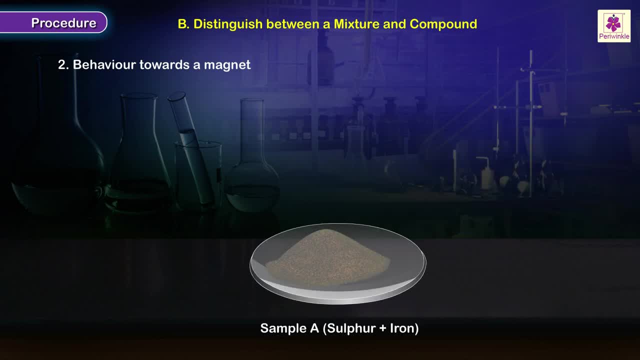 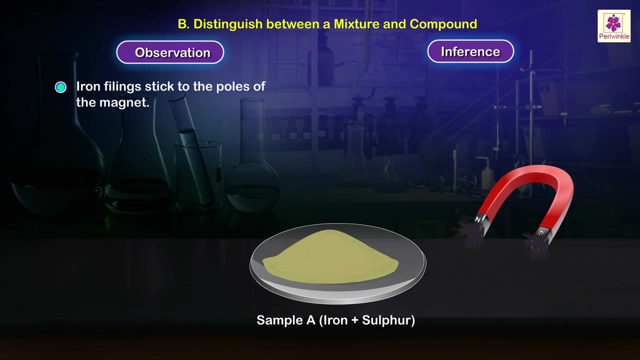 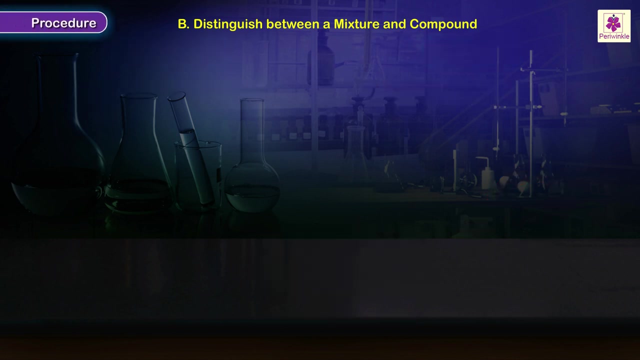 Place a spoonful of sample A on a watch glass. Slowly move the magnet through the mixture. Observation and inference: Iron filings stick to the poles of the magnet. Iron in the mixture retains its magnetic property. Procedure: Place a spoonful of sample B on a watch glass. 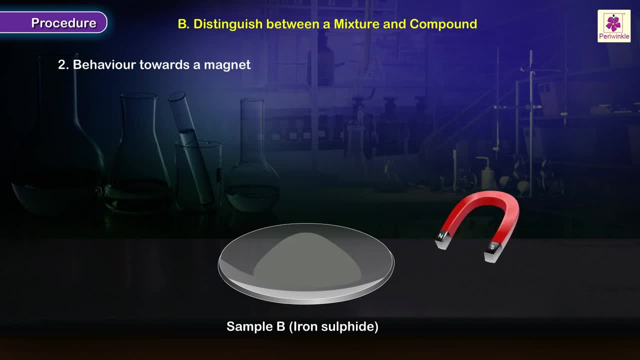 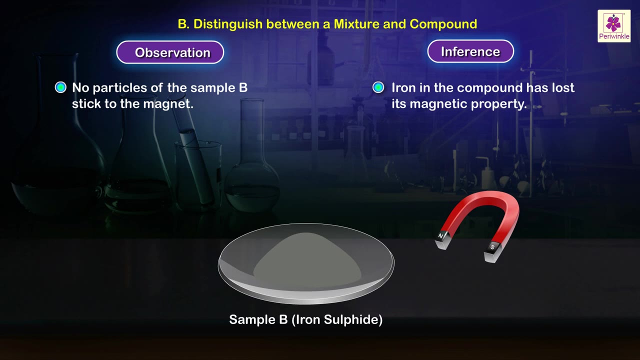 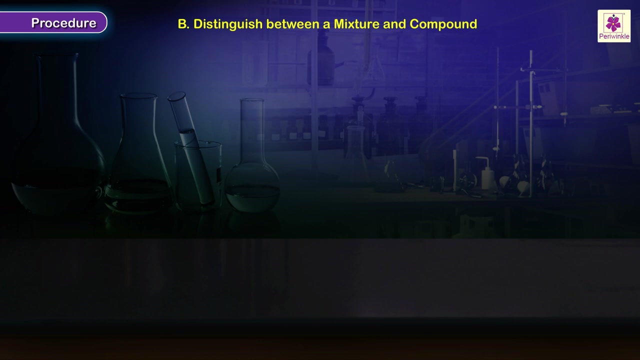 Slowly move the magnet through the powder. Observation and inference: No particles of the sample B stick to the magnet. Iron in the compound has lost its magnetic property Procedure to distinguish between a mixture and compound on the basis of their behavior towards carbon disulfide. 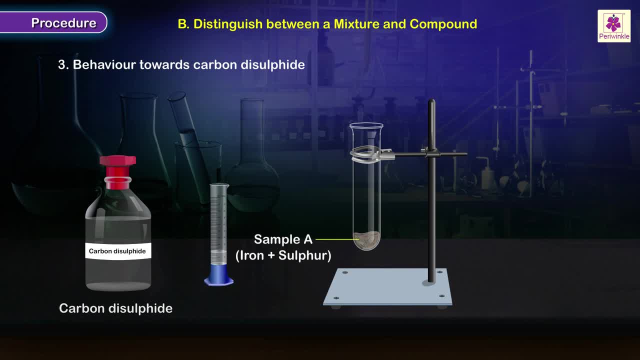 Take a small quantity of sample A in a clean dry test. you add about one to two milliliter of carbon disulfide to the test you and shake it well To get the resultLAB illusion of predictable imbalances. let's look at three free tests. 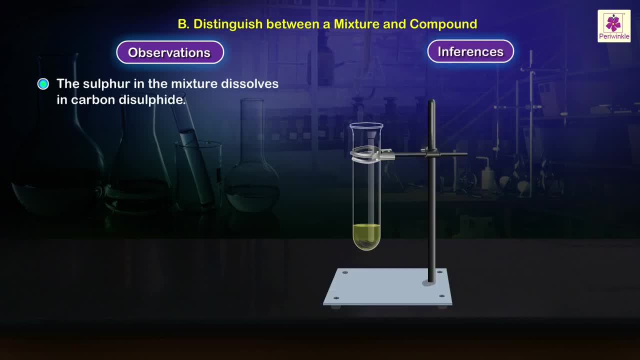 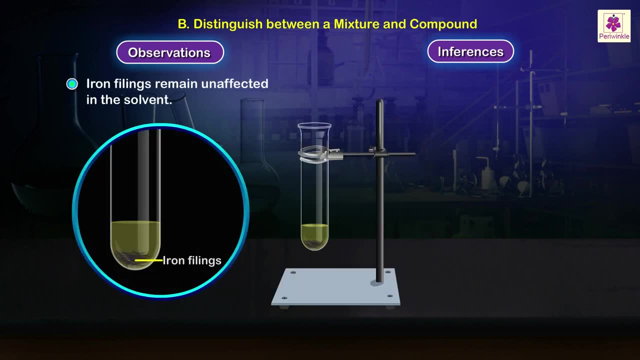 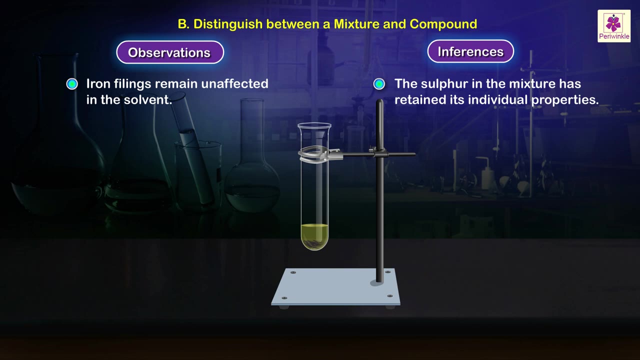 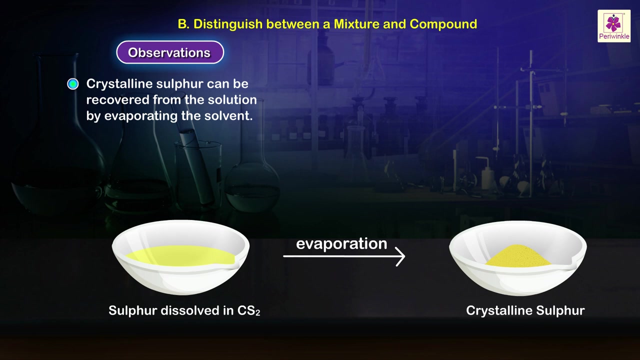 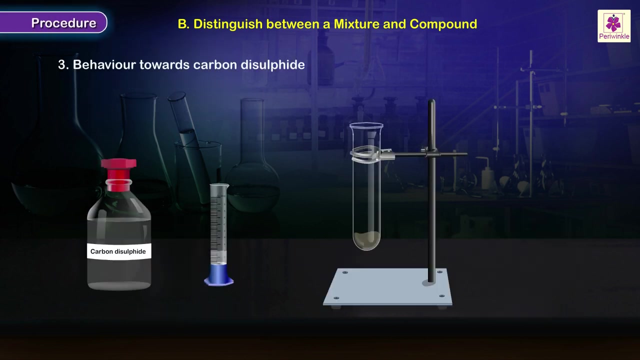 observations and inferences. the sulfur in the mixture dissolves in carbon disulfide. iron filings remain unaffected in the solvent. the sulfur in the mixture has retained its individual properties. crystalline sulfur can be recovered from the solution by evaporating the solvent procedure. take a small quantity of sample B in a clean, dry test tube. add 1 to 2 milliliter of. 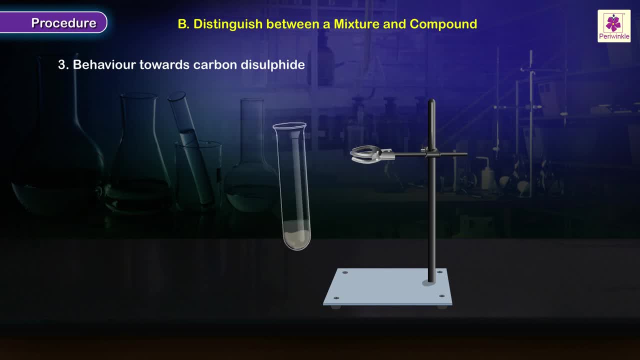 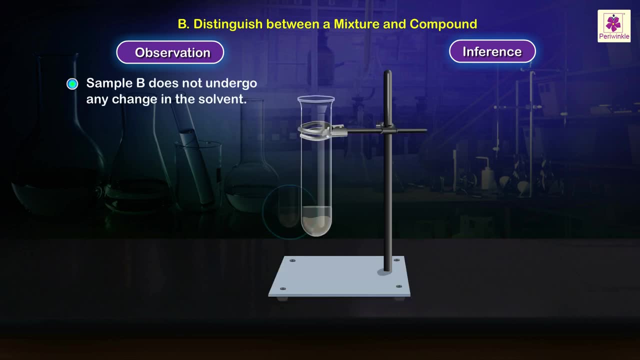 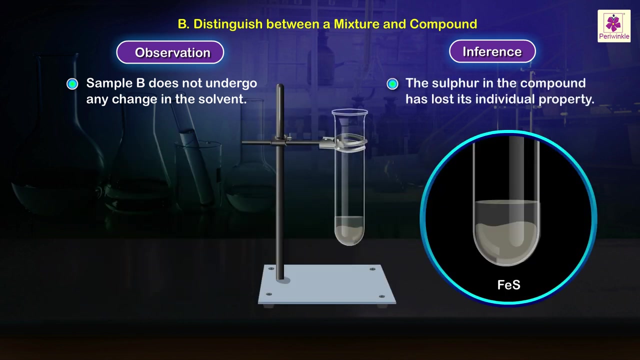 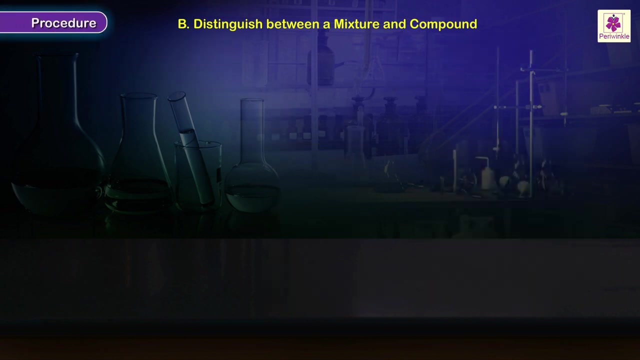 carbon disulfide to the test tube and shake it well. observation and inference. sample B does not undergo any change in the solvent. the sulfur in the compound has lost its individual property procedure to distinguish between a mixture and compound on the basis of the effects of heat. a part of the sample A was already heated to. 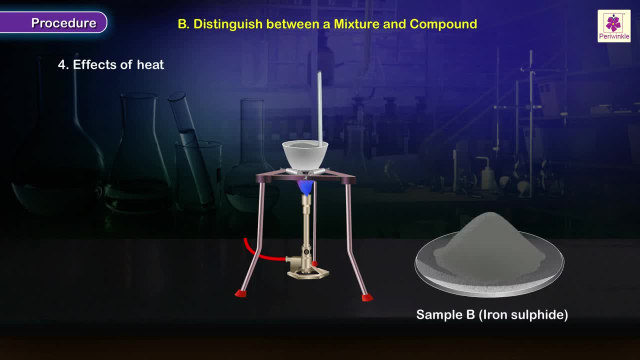 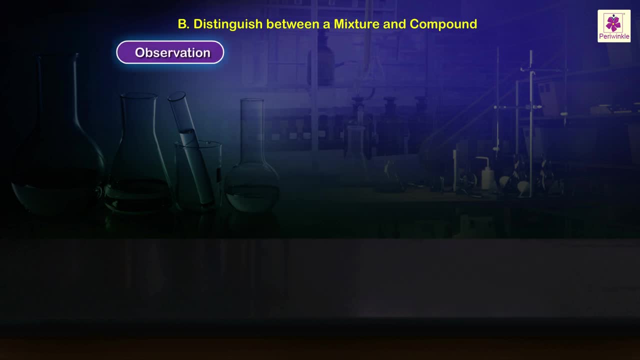 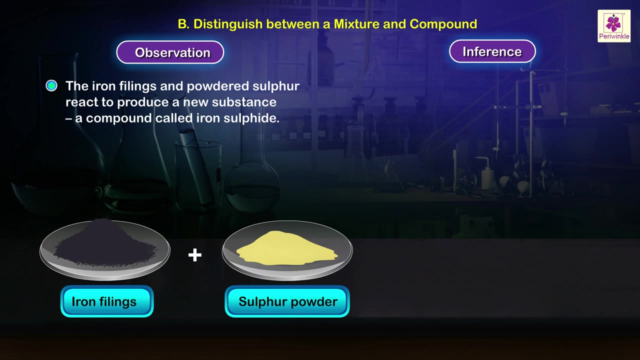 prepare the compound iron sulfide. hence it is not necessary to heat the mixture again. observation and inference: the iron filings and powdered sulfur react to produce a new substance, a compound called iron sulfide. heat converts the mixture of iron and sulfur into a compound iron sulfide procedure. take a: 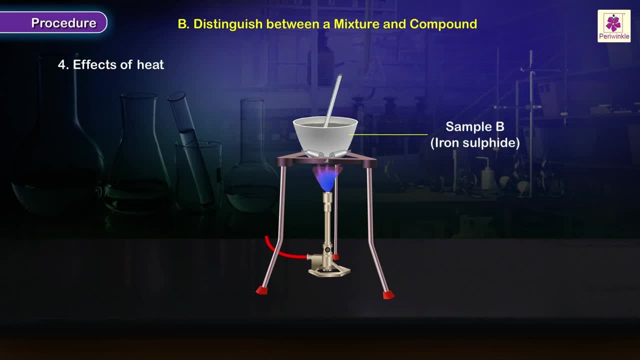 small quantity of powerful sulfur and baking soda in a hand mixer to make both for surface and fluid nitrogen and sulfur behind sulfur and baking soda forever by familia procedure. take a small quantity of sample Powdered iron sulphide in a crucible and heat it strongly on a gas burner. 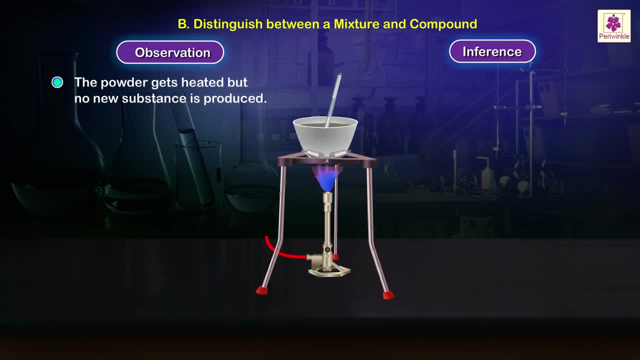 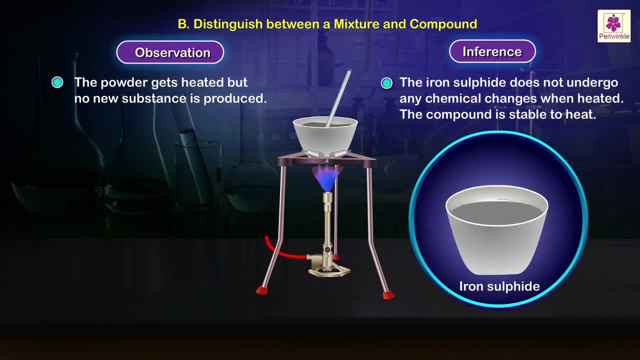 Observation and inference. The powder gets heated but no new substance is produced. The iron sulphide does not undergo any chemical changes when heated. The compound is stable to heat. Conclusion Or results.